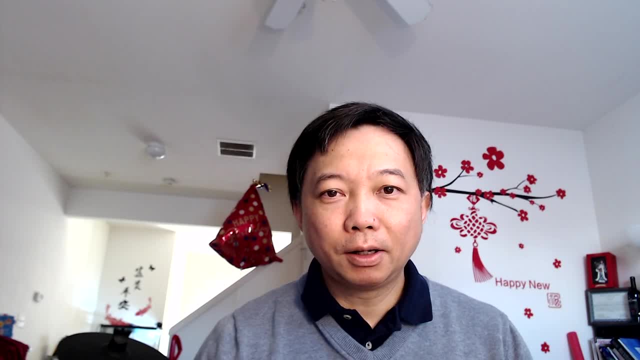 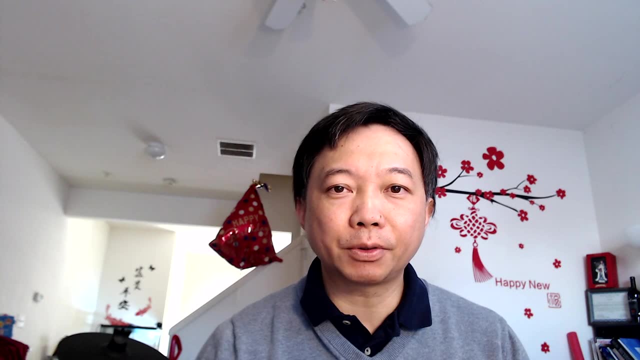 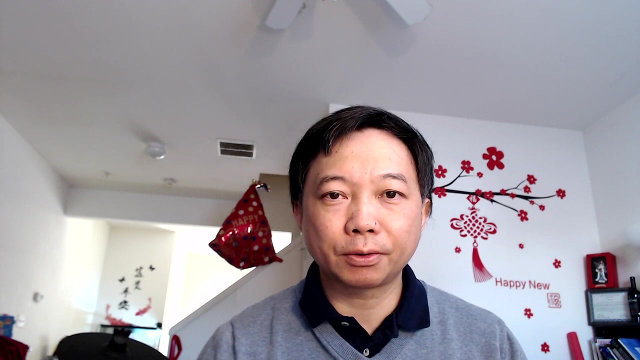 Hi, I'm Bob. Today let's learn Chapter 13, Game Theory. In this chapter, we will learn the static games and the dynamic games. We will learn the basic concepts in game theory, such as payoffs, strategy and Nash equilibrium. 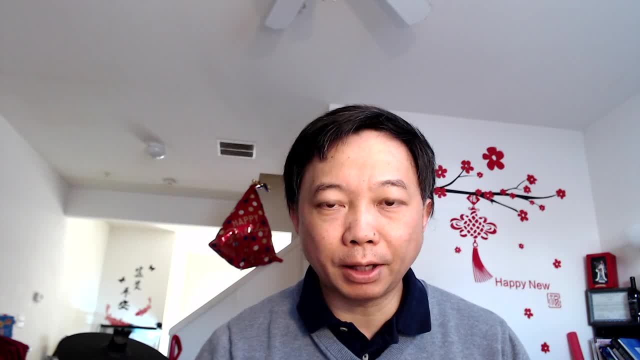 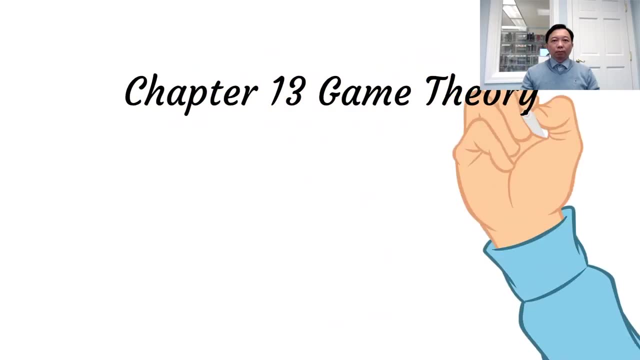 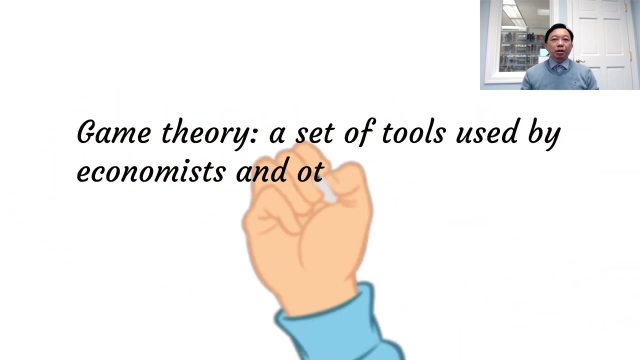 We will use the normal form, representation and the game tree to analyze a game. Game theory is a set of tools used by economists to analyze strategic decision-making. Game theory has many practical applications. Economists use it to study how oligopolistic firms set prices, quantities and advertising levels. 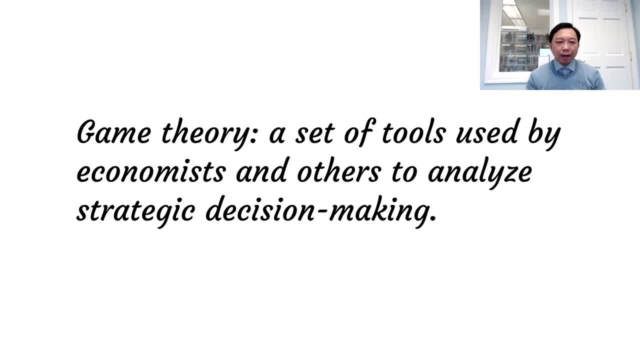 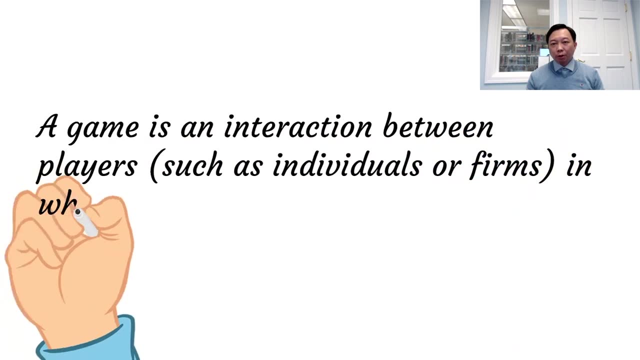 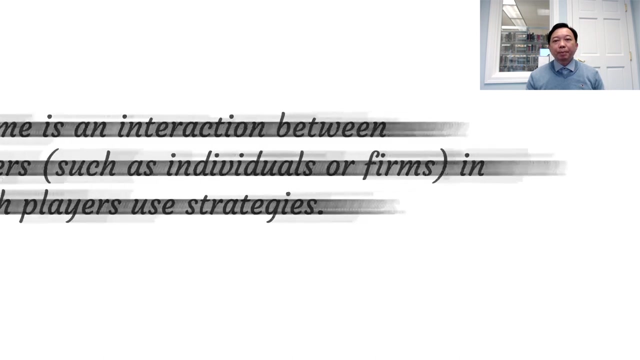 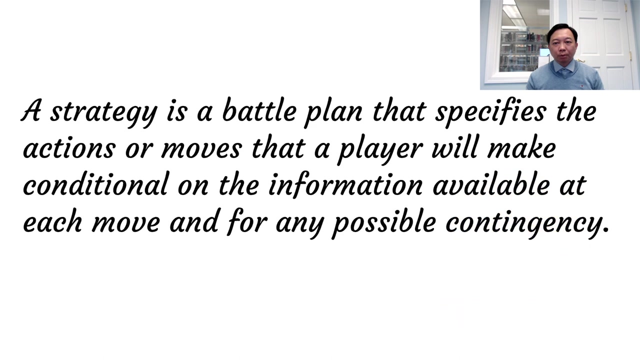 Bargaining between unions and management, or between companies, or between the buyer and seller, and for many other economic interactions. A game is an interaction between players, such as individuals or firms, in which players use strategies. A strategy is a plan that specifies the actions or moves that a player will make, conditional on the information available and for any possible contingency. 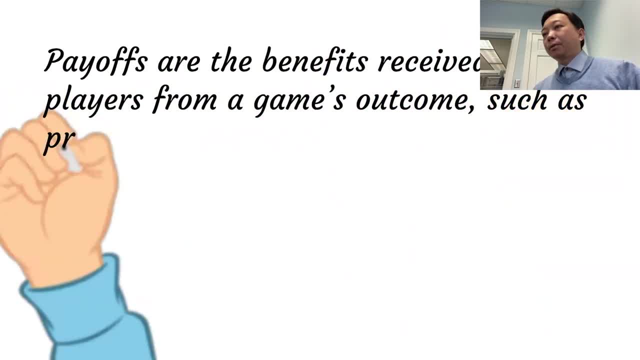 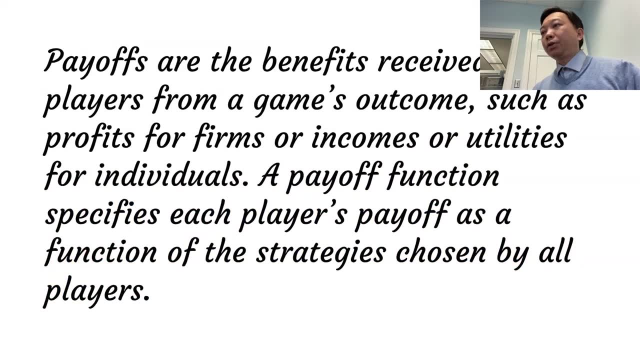 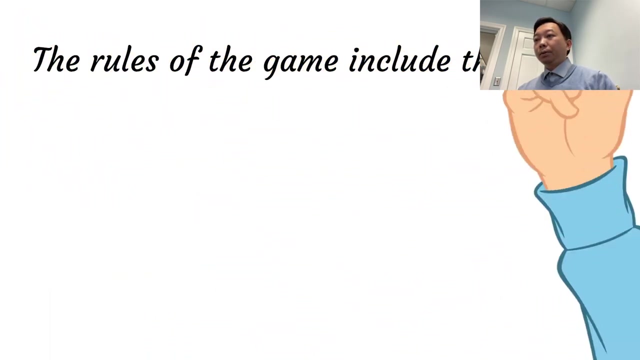 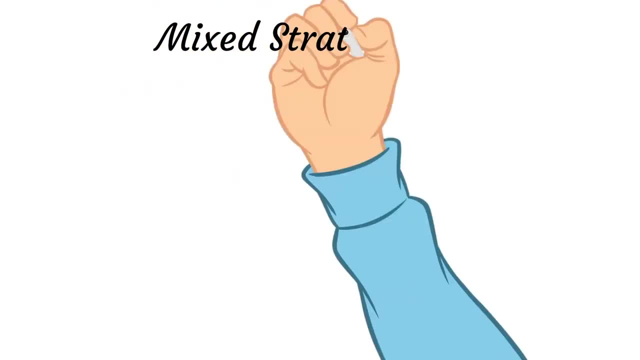 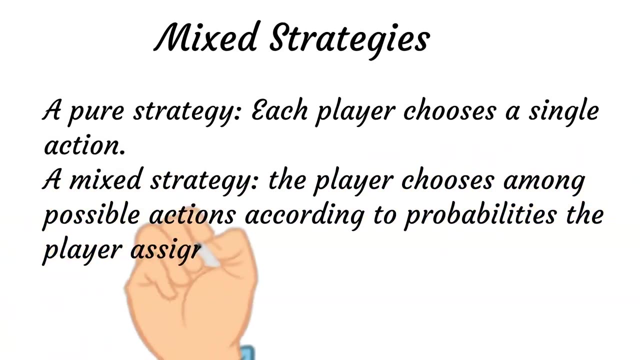 If the players have complete information. the strategies and payoffs of the game are common knowledge. If a firm uses a pure strategy, it chooses a single action. In addition to using a pure strategy, a firm may employ a mixed strategy In which the player chooses among possible actions according to probabilities. a player 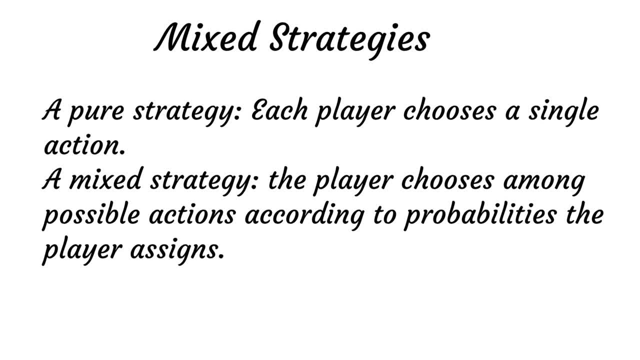 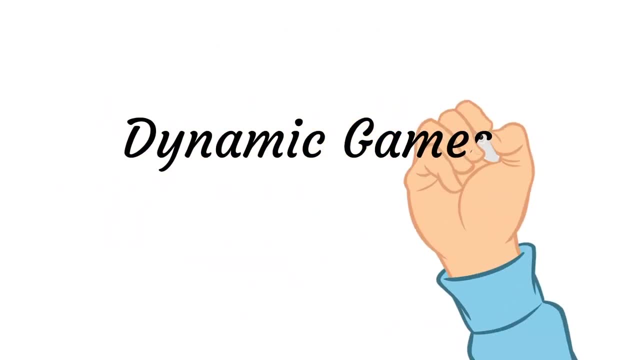 assigns. A pure strategy assigns a probability of 1 to a single court. A pure strategy assigns a probability of 1 to a single court, whereas a mixed strategy is a probability distribution over actions. A major difference between static games and dynamic games is that 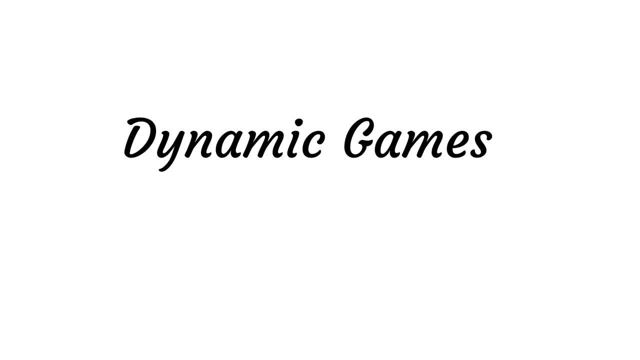 dynamic games requires to distinguish between strategies and actions. An action is a single move that a player makes at a specified time, such as choosing an output level or price. A strategy is a plan that specifies the full set of actions that a player will make throughout the game and may involve actions. 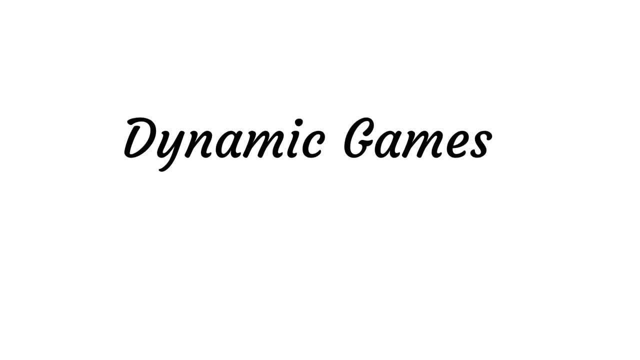 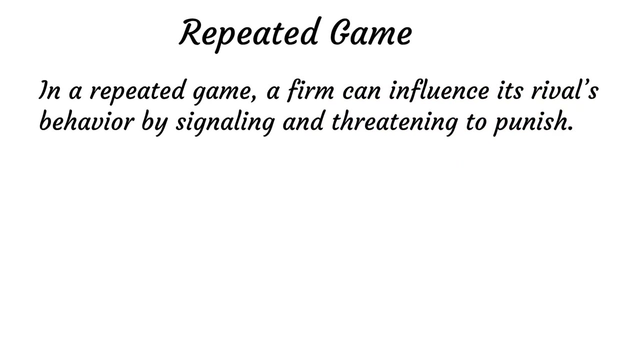 that are conditional on prior actions of other players or on additional information available at a given time. We consider two types of dynamic games. We start with a repeated or multi-period game in which a single-period simultaneous move game, such as the prisoner's dynamic game, is repeated at least twice. 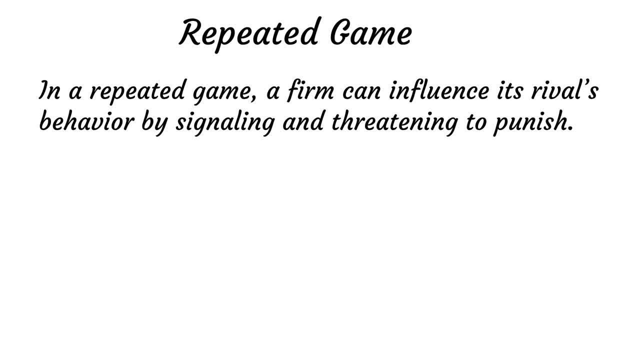 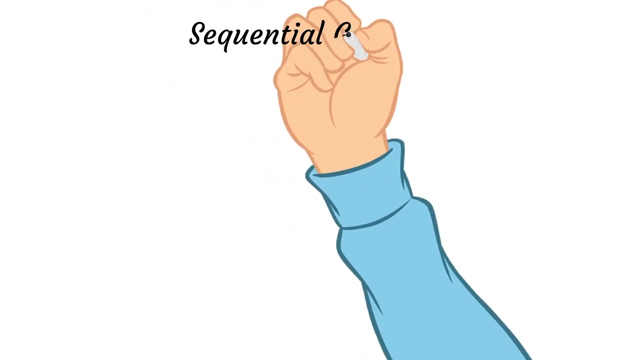 and possibly many times In a repeated game. a firm can influence its rival's behavior by signaling or threatening to punish. Collusion or cooperation is therefore more likely in a game that will continue forever or one that will end at an uncertain time. In a sequential game, we can use an extensive form diagram. 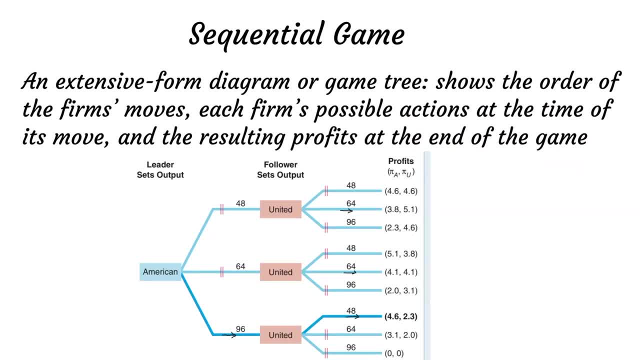 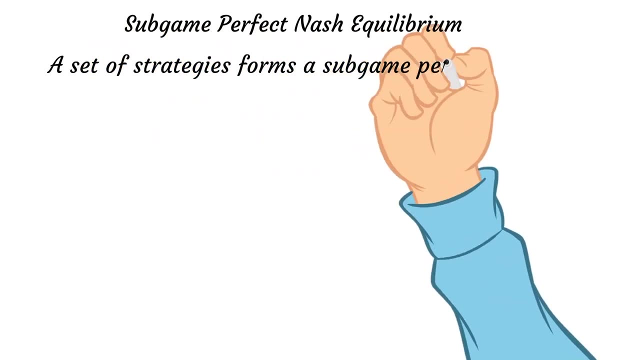 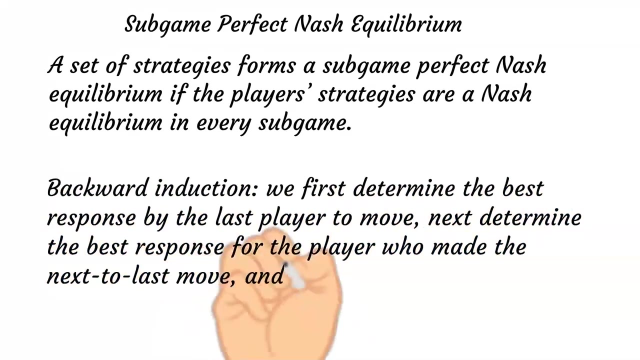 or game tree to show the order of the firm's moves, each firm's possible actions at the time of its move and the resulting profits at the end of the game. A set of strategies forms a sub-game-perfect Nash Equilibrium. if the player's strategies are Nash Equilibrium in every sub-game. 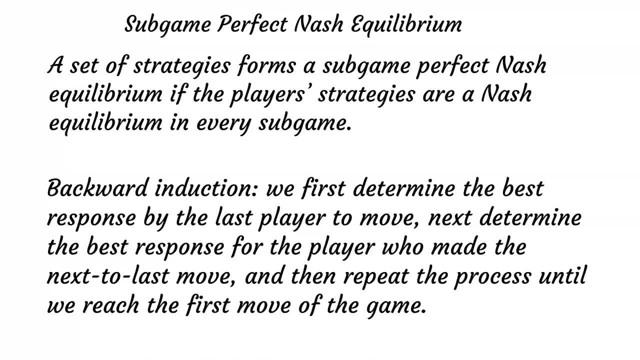 We can solve for the sub-game-perfect Nash Equilibrium using backward induction, where we first determine the best response by the last player to move, next determine the best response for the player who makes the next to last move, and then repeat the process until we reach the first move of the game. 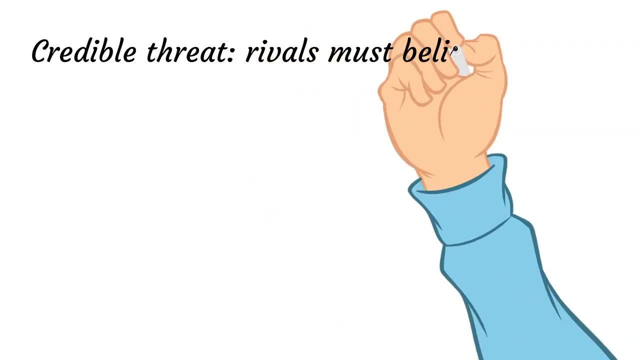 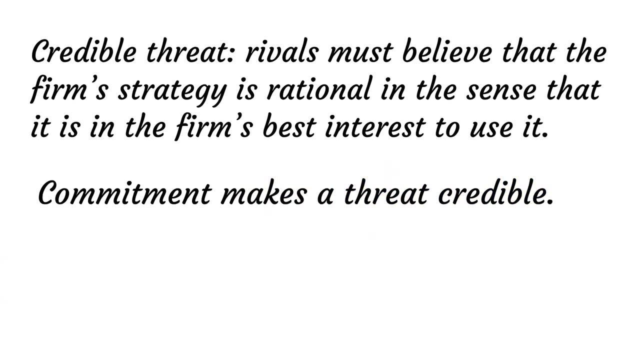 For a firm's strategy to be a credible threat, rivals must believe that the firm's strategy is rational in the sense that it is in the firm's best interest to use it. A firm may be able to make its threatened behavior believable if it acts before the other. 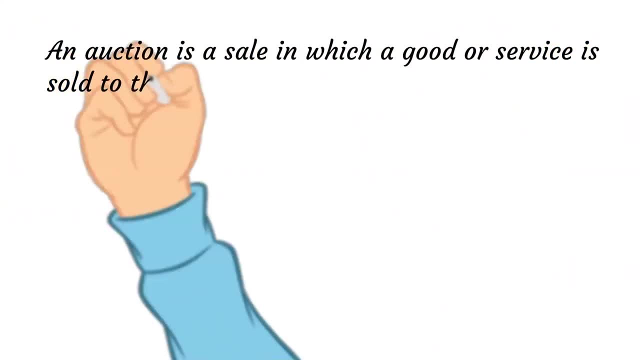 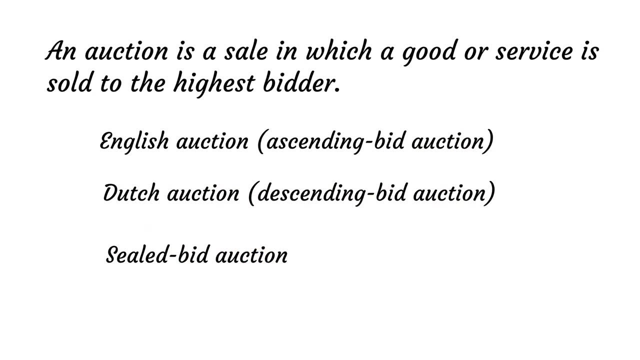 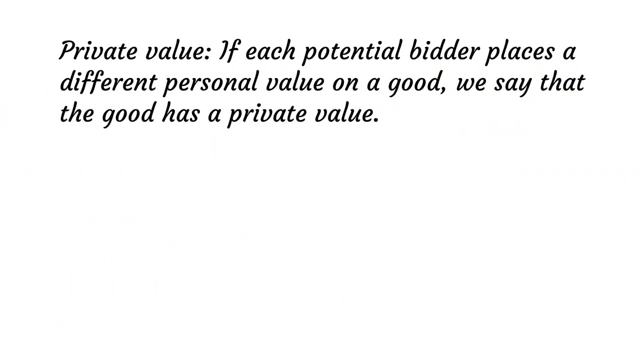 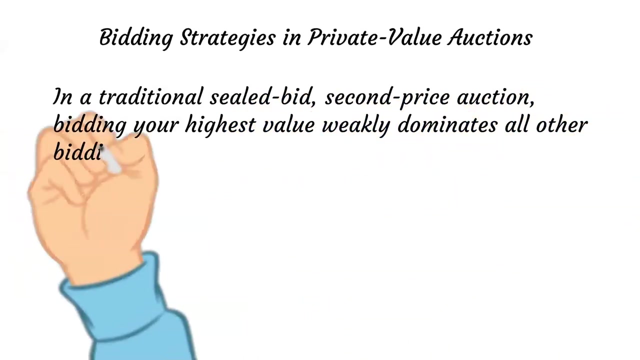 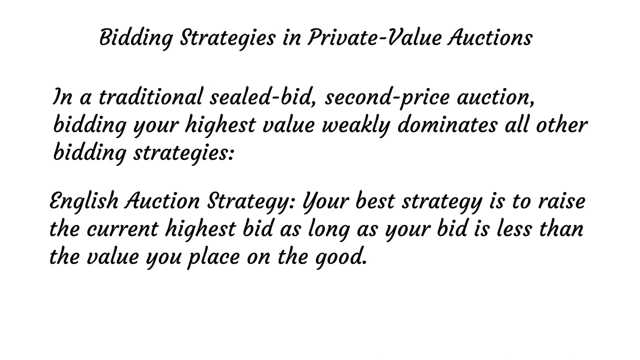 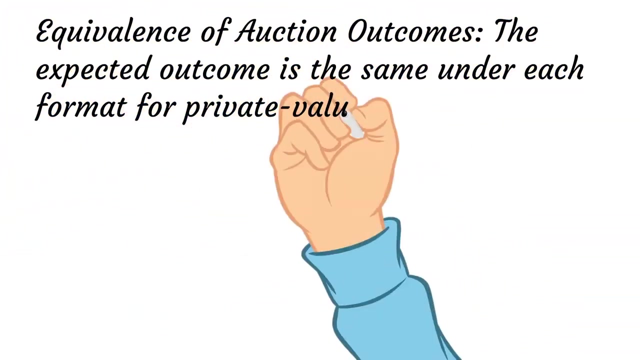 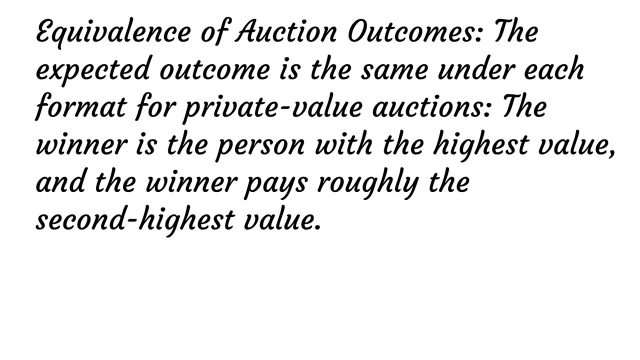 An option is a cell in which a good or service is sold to the highest bidder. Virtually all options are variants of the English option, the Dutch option and the Suebid option. We normally assume that people are rational in the sense that they optimize. 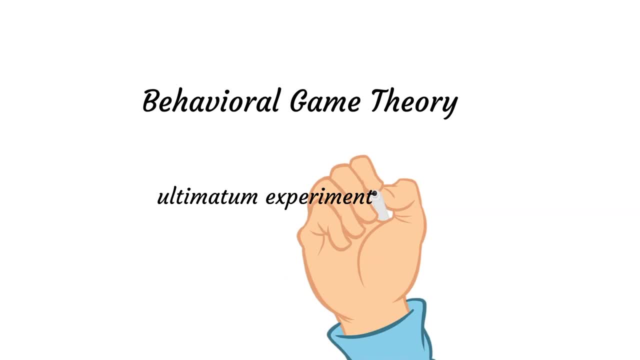 they optimize using all available information. However, they may be subject to psychological biases and may have limited powers of calculation. that causes them to act irrationally. Such possibilities are the domain of behavioral economics, which cease to augment the rational economic model so as to better understand and predict economic decision-making.